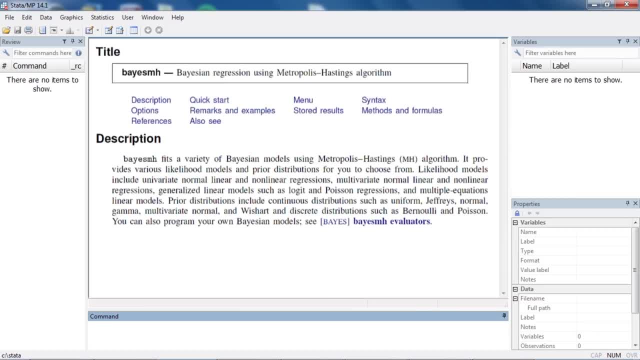 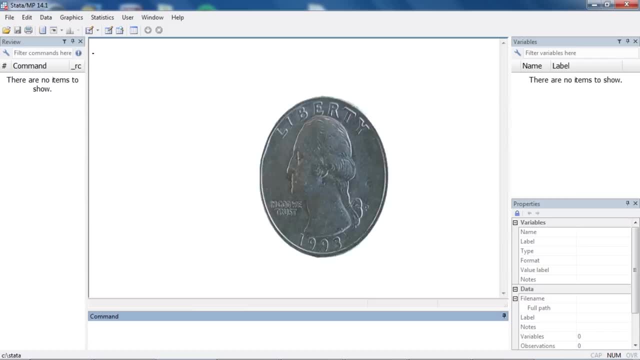 algorithm. In the interest of brevity, I'm going to omit some details and I strongly encourage you to read the manual before using MCMC in practice. Let's continue with the coin toss. example from Part 1.. We are interested in the posterior. 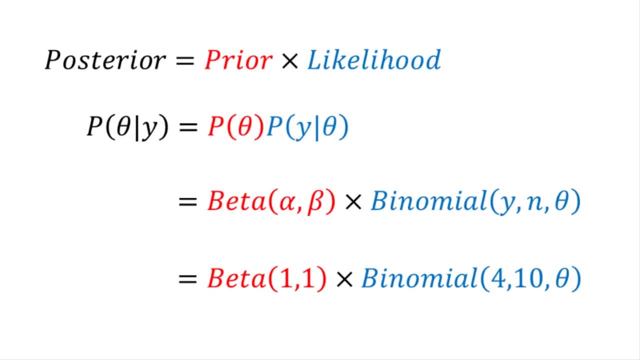 distribution of the parameter theta, which is the probability that a coin toss results in heads. Our prior distribution is an uninformative or flat beta distribution with parameters 1 and 1.. And we will use a binomial likelihood function to quantify the data from our experiment. 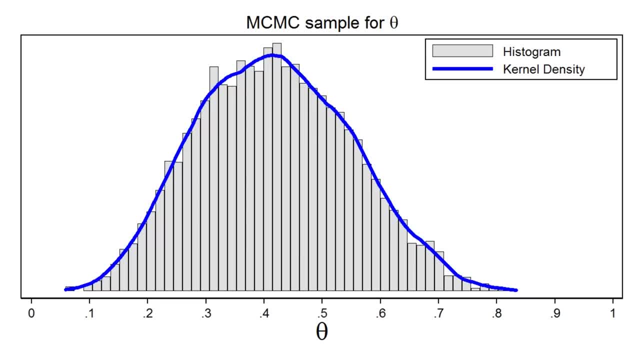 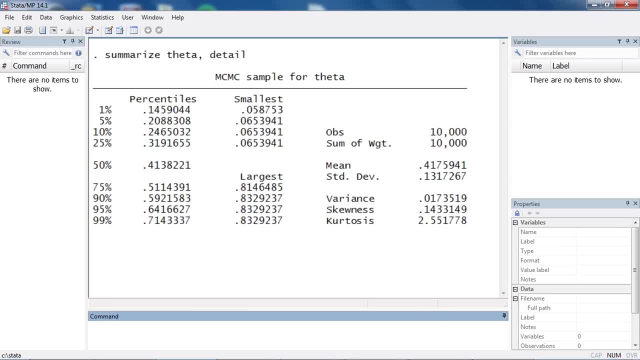 which resulted in 4 heads out of 10 tosses. We can use MCMC with the Metropolis-Hastings algorithm to generate a sample from the posterior distribution of theta. We can then use this sample to estimate things such as the mean of the posterior distribution. 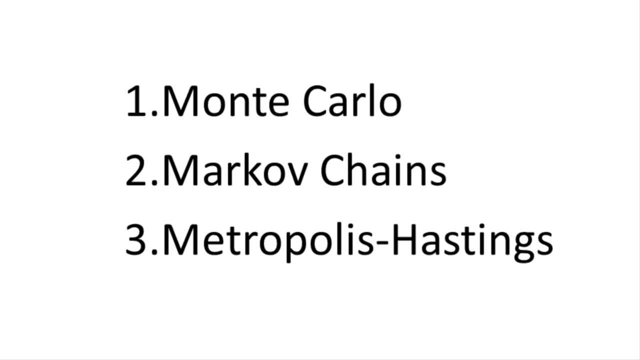 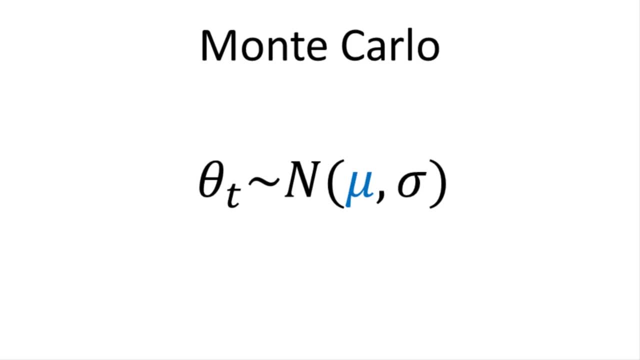 There are three parts to this technique: the Monte Carlo part, Markov chains and the Metropolis-Hastings algorithm. The term Monte Carlo refers to methods that rely on the generation of random numbers. For example, I could generate a series of random numbers from a normal distribution with a mean of 0.5 and some arbitrary variance sigma. 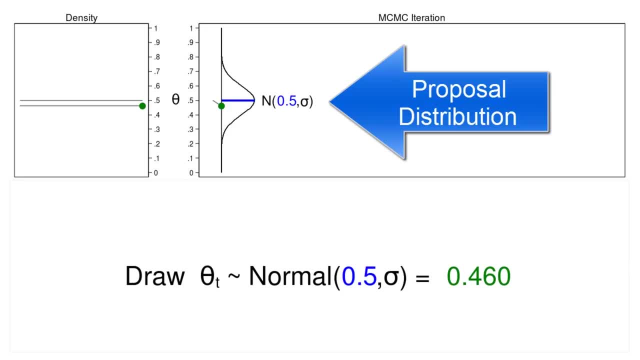 In this example, I'm going to refer to the normal distribution as the proposal distribution In the graph on the right. I'm going to shift the proposal distribution to the right each time I draw a value of theta. This graph is called a trace plot and it allows me to view: 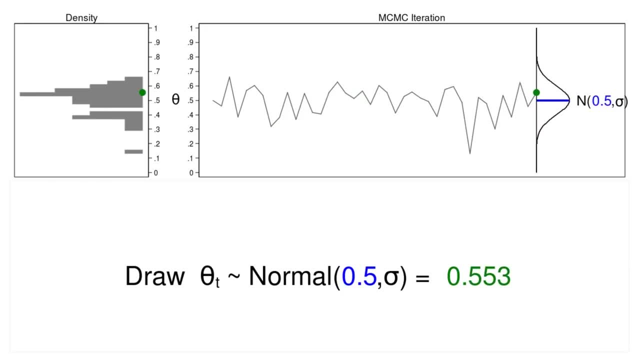 the values of theta in the order in which they were drawn. The density plot on the left is a histogram of the samples we have generated Here. I have rotated the density plot so that the theta axes for both graphs are parallel. If we were to generate 10,000 numbers, the 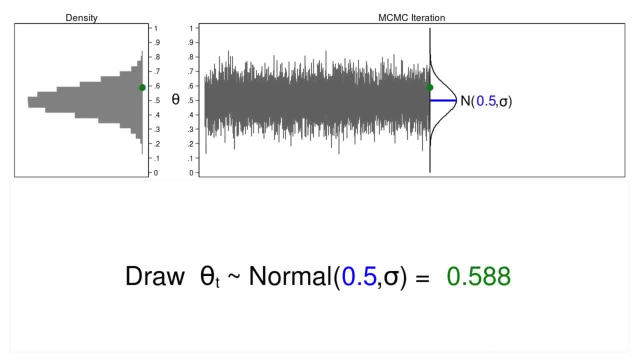 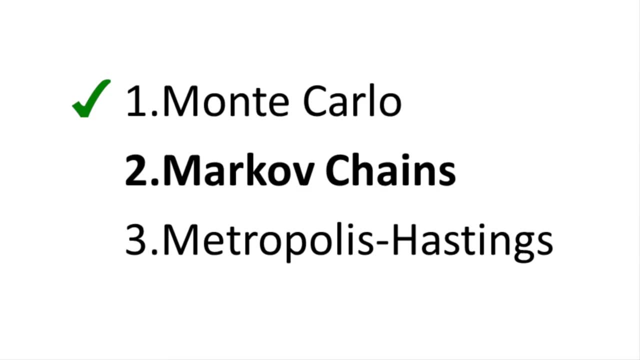 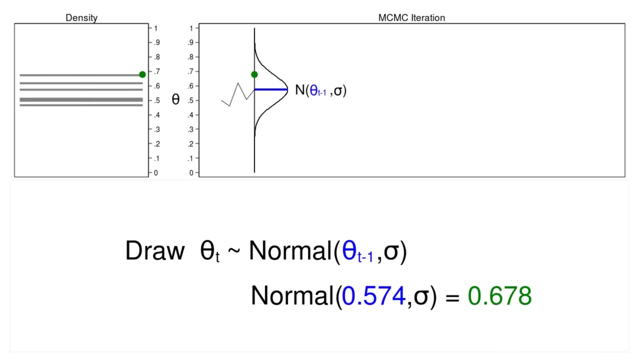 resulting density looks much like our proposal distribution. Note that the proposal distribution does not change from one iteration to the next. A Markov chain is a sequence of numbers where each number is dependent on the previous number in the sequence. In this example, each value of theta is drawn from a normal proposal distribution with a mean equal to. 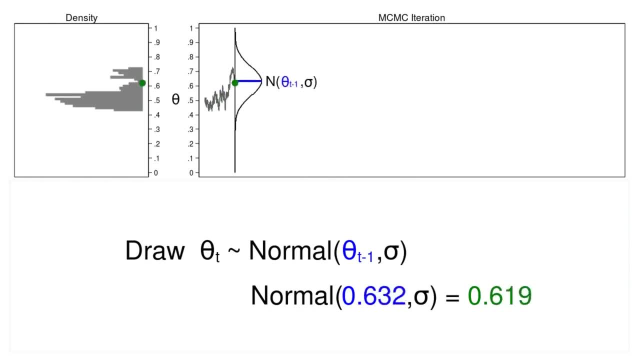 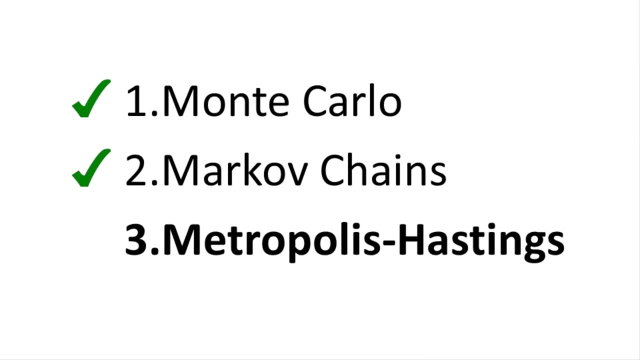 the previous value of theta. If we generate 10,000 numbers using Markov chain Monte Carlo, the trace plot of theta appears to wander and is often called a random walk. Note that the resulting density plot does not resemble the proposal distribution. The Metropolis-Hastings algorithm is used to decide which proposed values of theta to 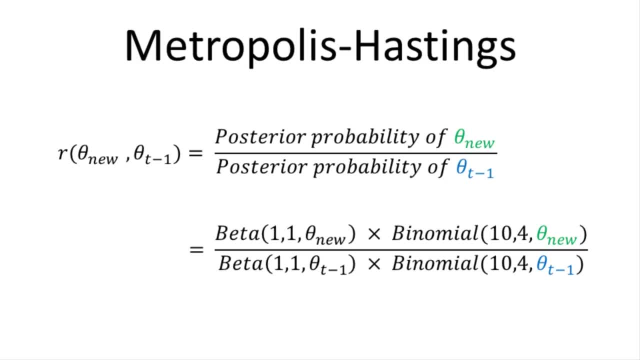 accept or reject. We begin by calculating the posterior probability using the newly generated value of theta. We also calculate the posterior probability using the previous value of theta. Notice that we don't have to know the functional form of the posterior distribution. We simply multiply the prior distribution and the likelihood function. 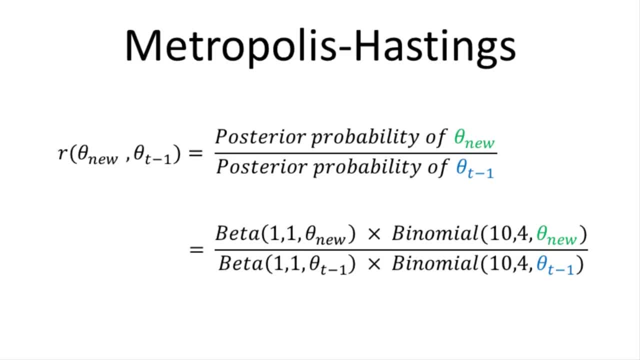 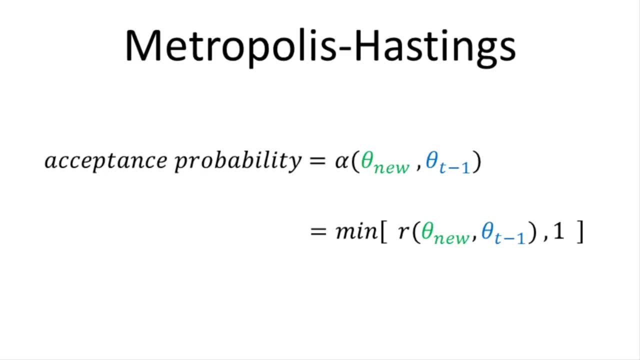 If the posterior probability is greater for the new value of theta, the ratio of the probabilities will be greater than 1 and we will always accept the new value of theta. If the posterior probability is greater for the previous value of theta, we will not necessarily discard. 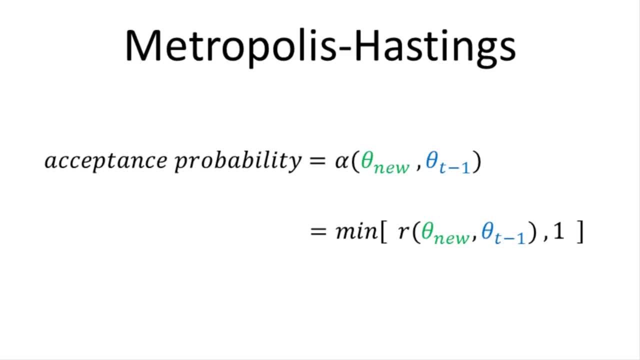 the new value of theta. We can treat ratios less than one as an acceptance probability. then we can draw a uniform random number and keep the new value of theta if the random number is less than the acceptance probability. Otherwise we discard the new value of theta. and can use this algorithm to decide the function from the question type of the answer. On the top of the calculator we find: 1. Prot, Consider theta as 0.. 아니야 omegaNone, o2k, 350n0O brains. 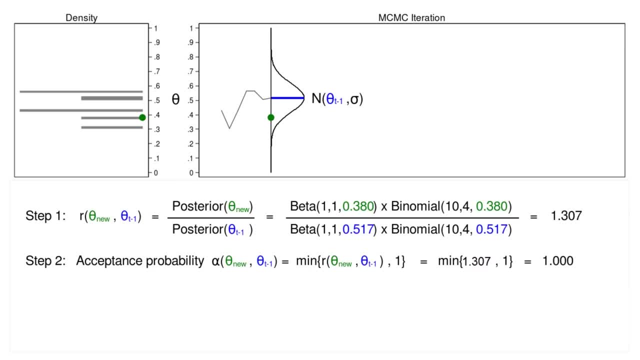 keep the previous value. Let's look at an example of how this works Here. the previous value of theta was 0.517 and we have drawn a new value of theta which equals 0.38 from our proposal distribution: The ratio of the posterior probabilities for the two values of theta. 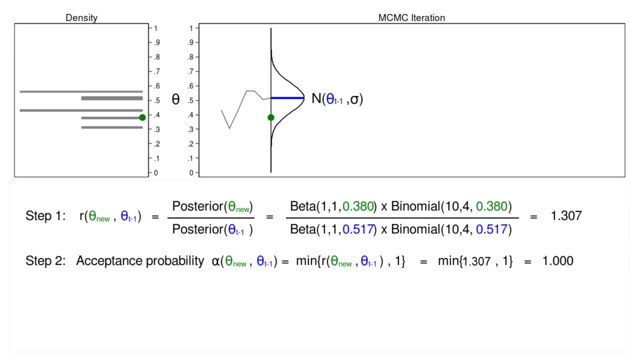 is equal to 1.307.. Since the ratio is greater than 1, the acceptance probability is 1 and we will keep the new value of theta. The new value of 0.38 becomes the previous value of theta and we draw a new value of theta from our proposal distribution, which equals 0.286.. 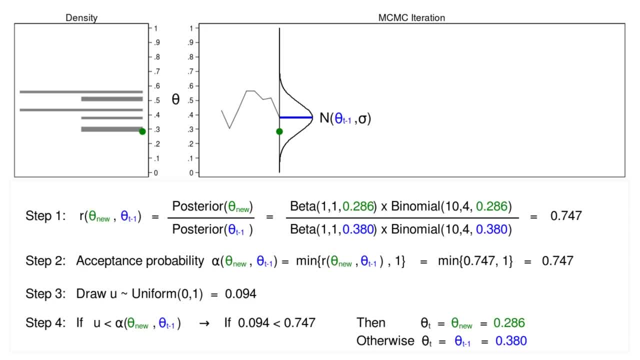 The ratio of the posterior probabilities, 0.747 becomes our acceptance probability and we draw a random number from a uniform distribution. The random number, 0.094, is less than the acceptance probability of 0.747, so we will keep the new value of theta. So the new value of 0.286 becomes: 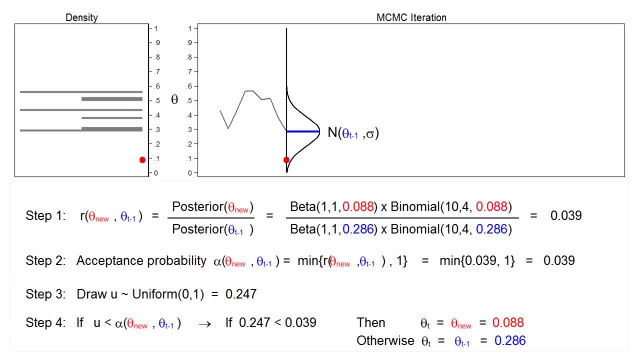 the previous theta and we draw a new theta from the proposal distribution, which equals 0.088.. The ratio of the posterior probabilities equals 0.039, which will be used as the acceptance probability. The random uniform number drawn in step 3 is larger than. 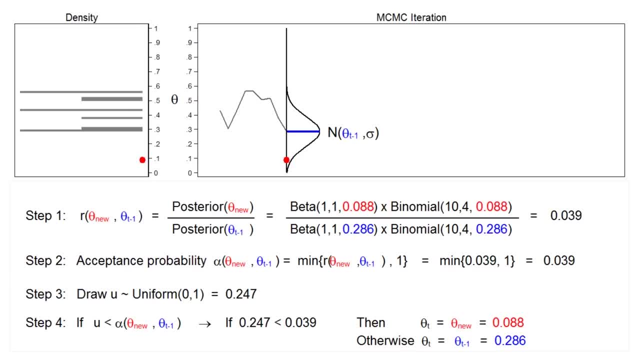 the acceptance probability. so we reject the new value of theta and keep the old value of 0.286.. I've displayed the new value of theta in red to indicate that it has been rejected. We can repeat this algorithm 10,000 times and notice that some proposed values. 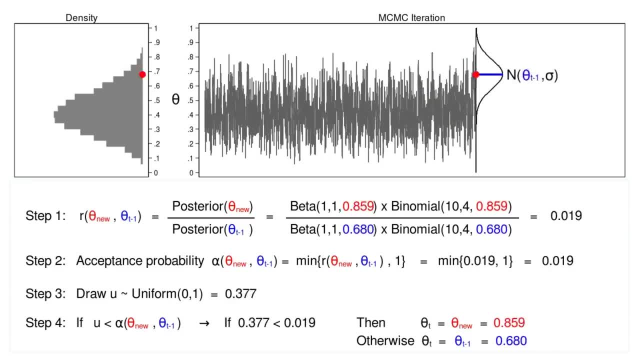 of theta are green, indicating that they have been accepted. The new values of theta are red, while others are red, indicating that they have been rejected. The result of this process is a sample from the posterior distribution. There are two issues with the Metropolis-Hastings. 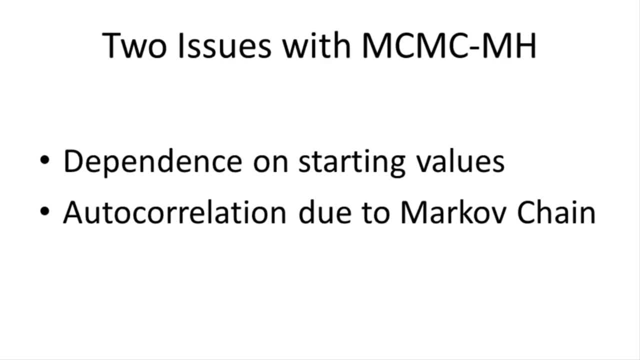 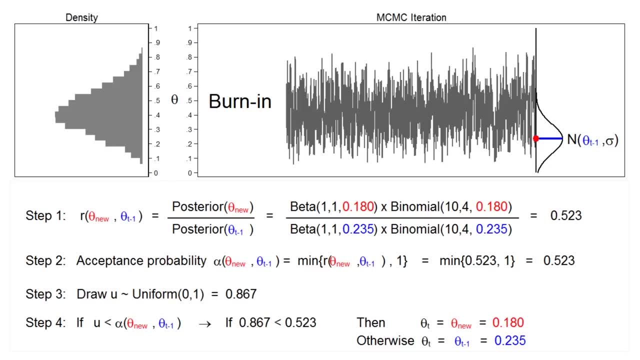 algorithm. First, the sample is dependent on the starting value. We can reduce the influence of the starting value by discarding the first part of the sample. This part of the sample is called the burn-in period. The burn-in period is the time it takes for the chain. 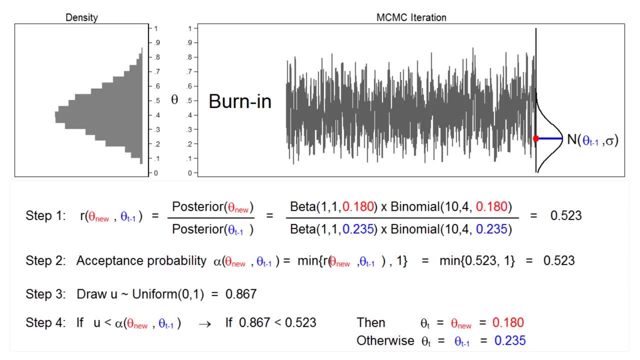 to stabilize so that it isn't drifting up or down over time. As a result, Stata discards the first 2500 values from the sample, but this default is arbitrary and you may want to use a different value after inspecting your trace plot. We. 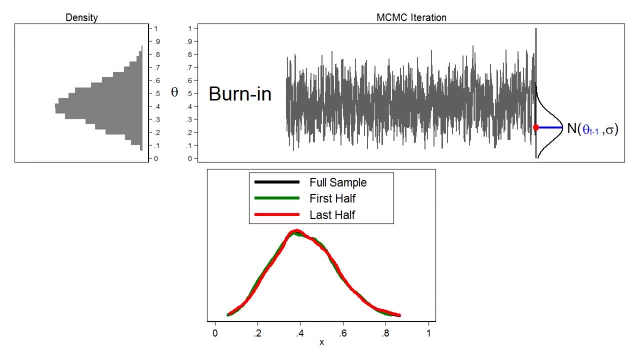 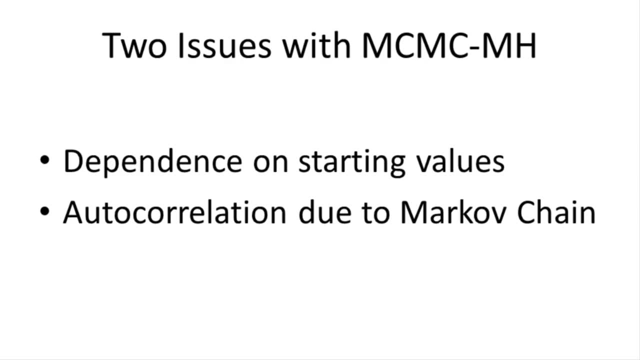 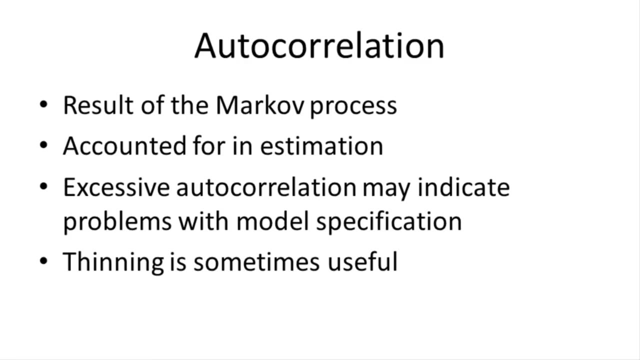 can also compare density plots of the first and last half of the sample with the full sample to look for differences. The second issue is that the values of theta are correlated because they are generated by a Markov process. This is normal and Stata accounts for the autocorrelation in its estimation algorithms. Excessive autocorrelation may 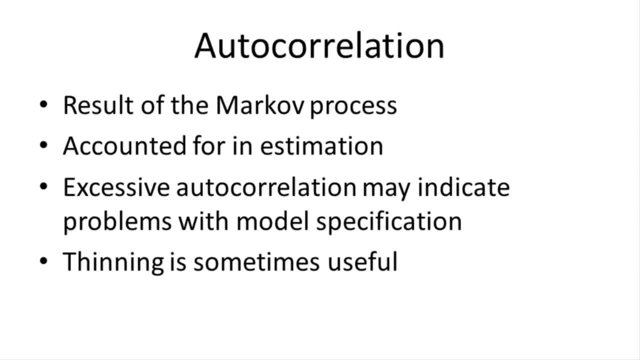 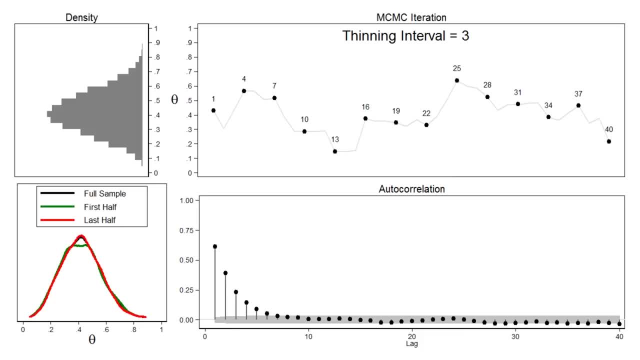 indicate problems with model specification and should be investigated further If the model is correctly specified. thinning is sometimes used to reduce autocorrelation. Thinning refers to the process of increasing the MCMC sample size and drawing samples at regular intervals. For example, we could generate a sample of 30,000 values and keep every third. 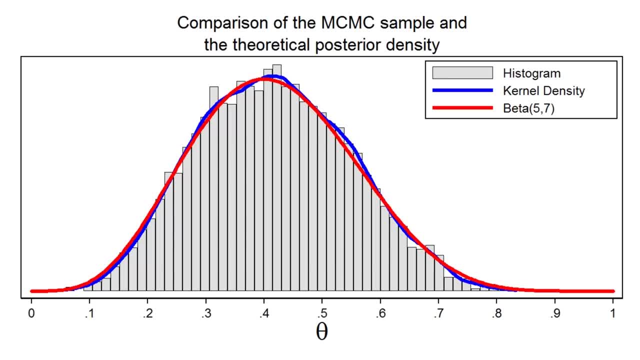 value. In this example, we know that the posterior distribution is a beta distribution with parameters 5 and 7.. This graph compares a histogram of the first and last half of the sample to the second half of the sample. In this case, our MCMC sample provides a very good approximation. 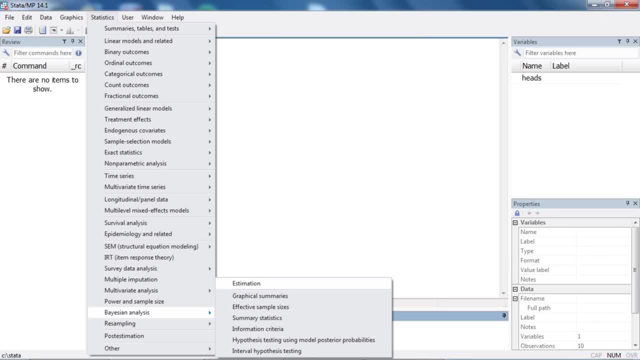 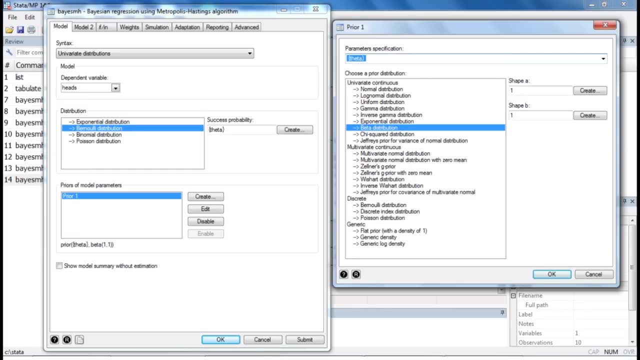 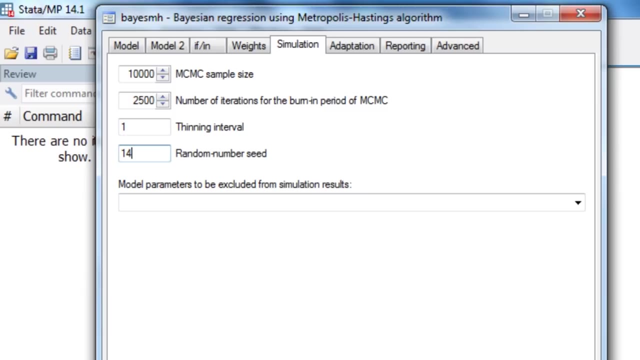 to the theoretical posterior distribution. So let's continue our coin toss. example: using Bayes-MH, We specified a beta distribution with parameters 1 and 1, along with a Bernoulli likelihood. Next, we can specify the size of our MCMC sample, the length of the burn-in period and the thinning interval in the simulation.